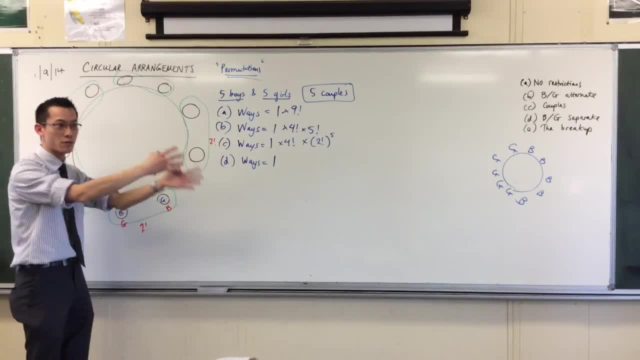 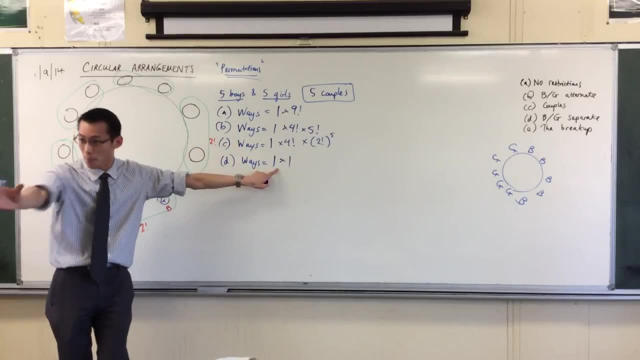 How many ways are there for me to chuck in the other group? Answer One way. There are only five seats left, right One. Okay, so I placed, say, the boys, There's a group of five. Then I placed the girls as a group of five. 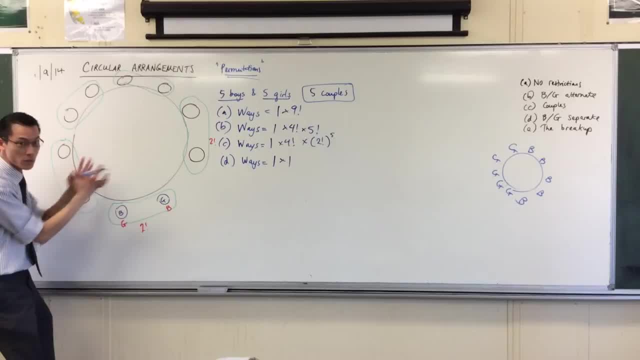 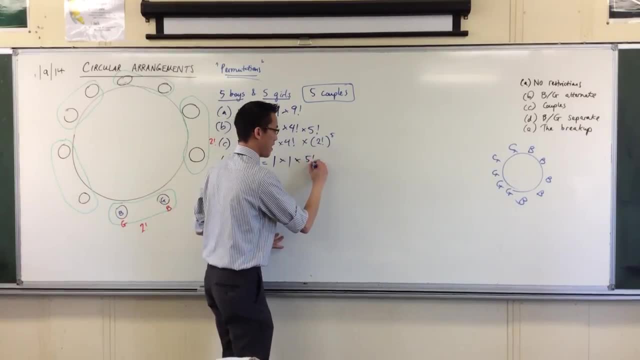 But then, just like in the couple situation, within those groups they can rearrange themselves right. So, for instance, how many ways can the boys rearrange themselves? Five factorial, And then the girls can also rearrange themselves into five factorial ways. okay, 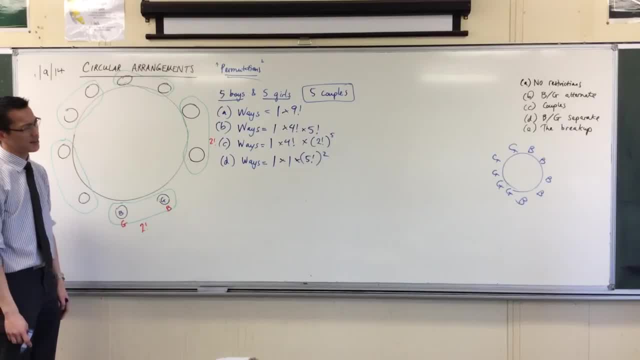 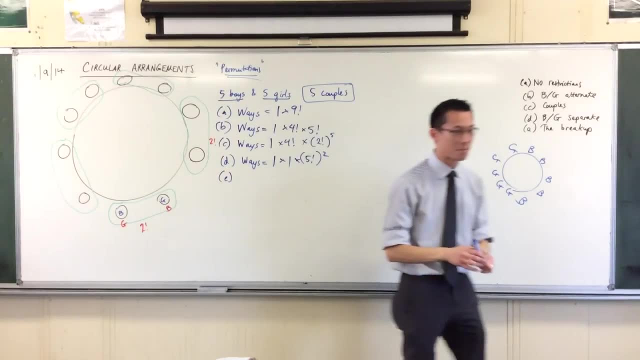 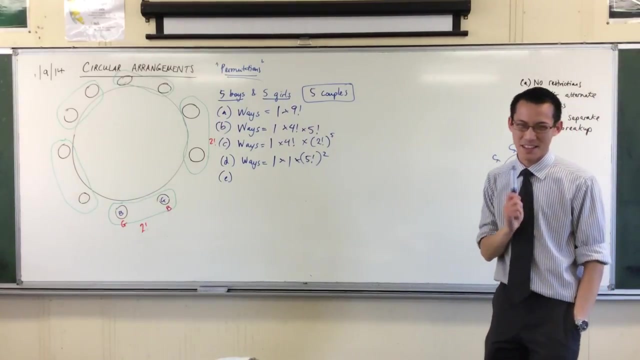 So there you go. Uh, 114,400? Something like that. Okay, Last situation: Oh, so sad A breakup. So let's go back to part C. We had five couples, right, Five couples, But suppose one of the couples breaks up. 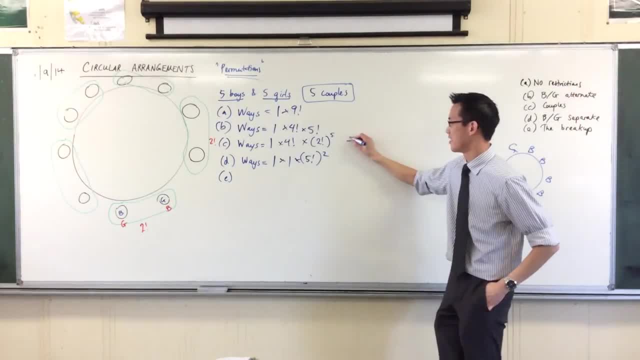 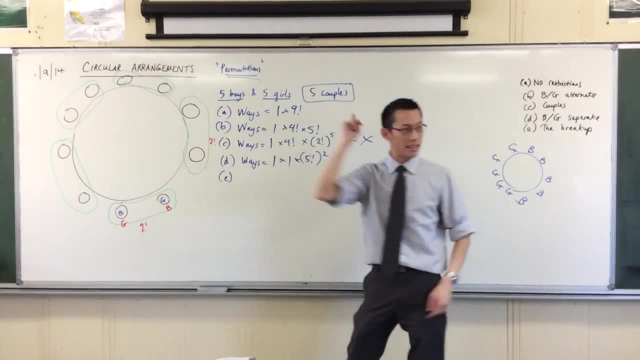 Okay, so we don't want to replay this one. That's a bad idea. okay, The four couples that are still together, they're okay, They're like this, right, But the other two, we want to keep them far apart. 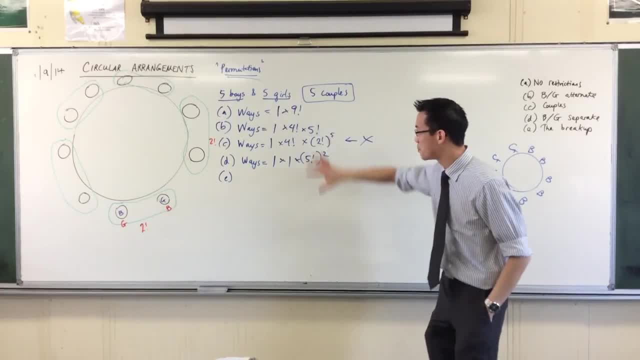 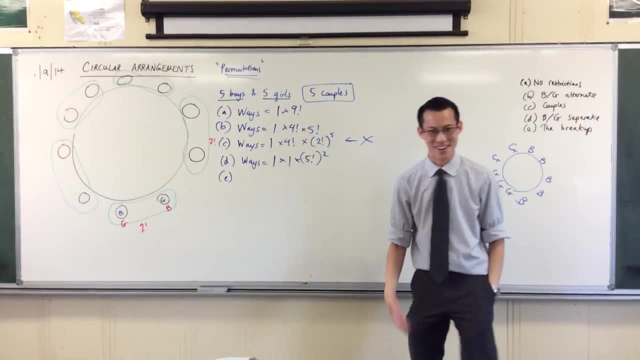 Okay, I'm going to pause. We've just built up all these approaches for doing it. Okay, I want you to have. Just boot him off the table, you know? Sorry, buddy, I want you to think about how you would do it and where you would start, right. 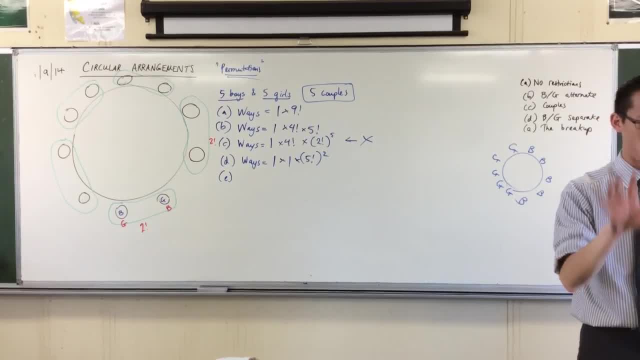 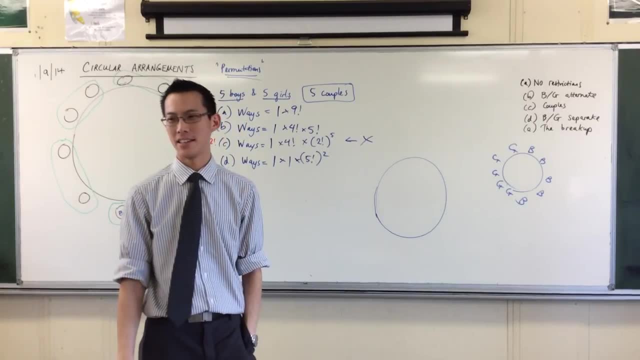 And then how you would explain how your way gets the right number of ways. And, by the way, I don't know who said it, but there's this really good quote that says: A problem well phrased is half solved. A problem well phrased is half solved. 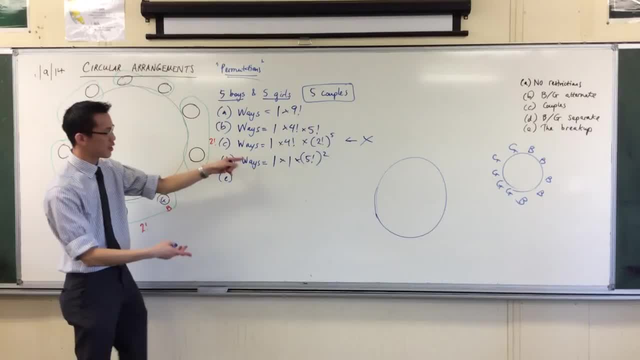 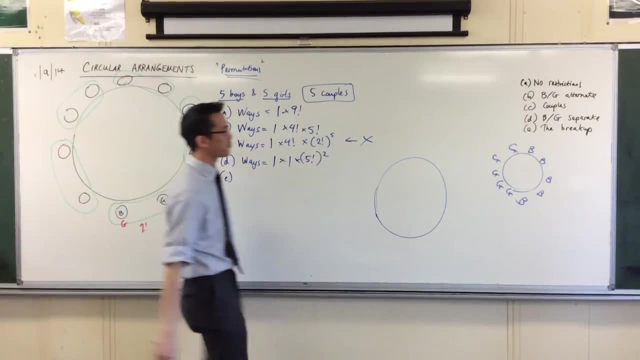 Because, if you phrase it the right way, it makes it very obvious what way you should proceed, And then the rest of it's just trivial, right? So here's the way I'm going to phrase it: It's a break up, right? 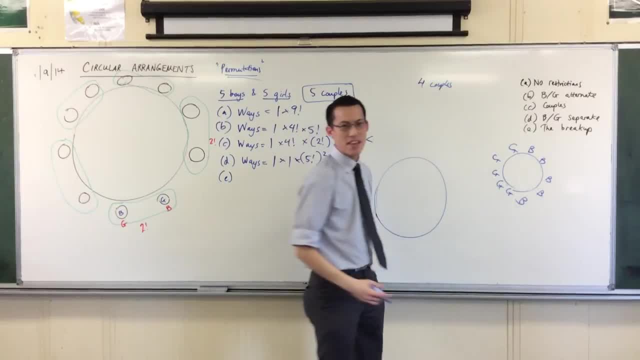 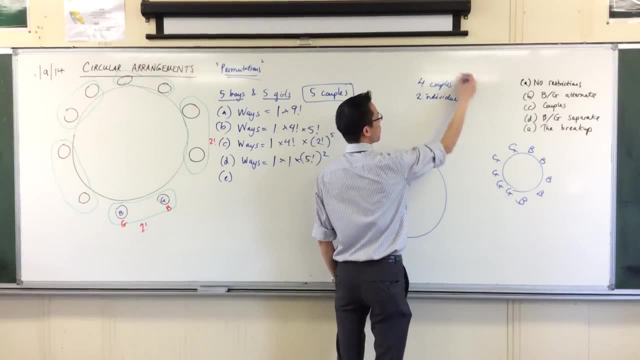 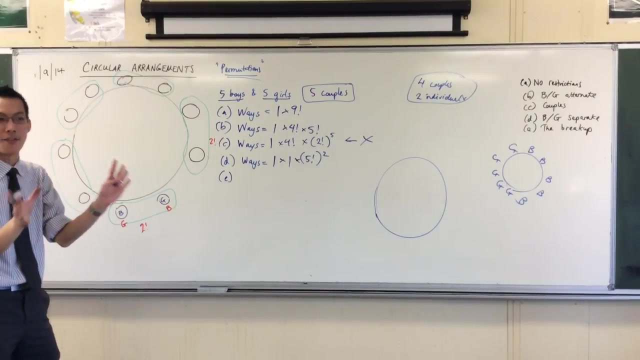 So you've got four couples and then you've got the other two, Two individuals, right? So these here, these are the things I need to place, Okay, and then I'll work out their internal rearrangements afterwards, okay. 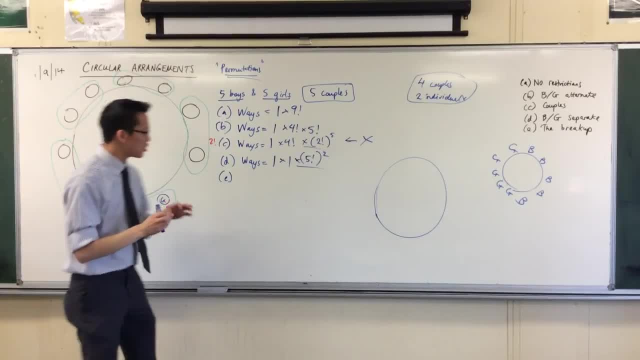 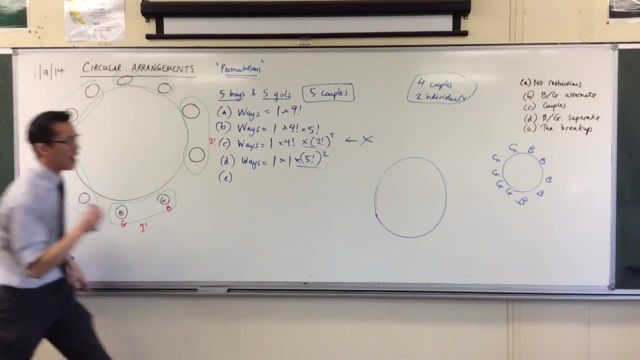 Just like I've been doing all the way through. Okay, So you know, in the case of the couples, how many couples did I have to place? I had five couples In the case of having all of the boys together and all the girls together. 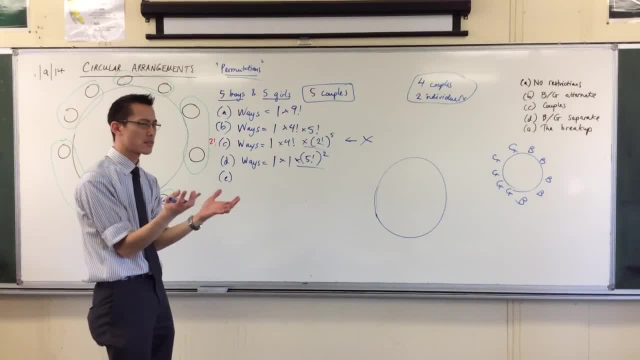 how many units objects did I need to place? I need to place two right, So I placed one, and then, because it's a circle, there's only one other place for the things to be okay. Now you have a look at this. 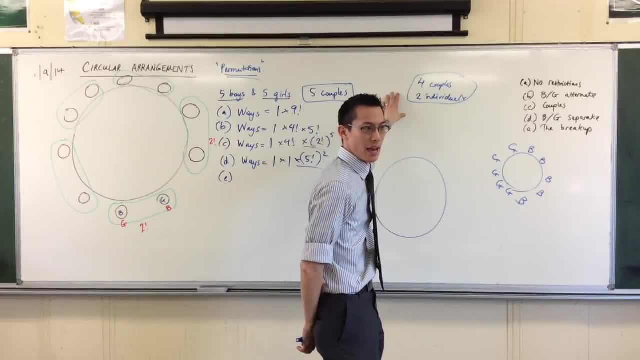 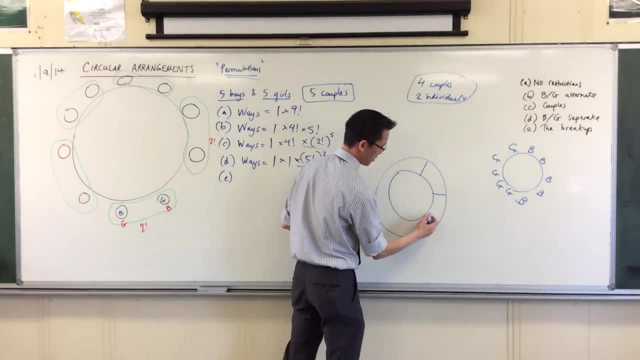 How many objects do I need to place? And the answer is six. okay, So I have six objects. So I'm going to put- I'll do it like this, because this you might find this a little more helpful- One, two, three, four, five, six, okay. 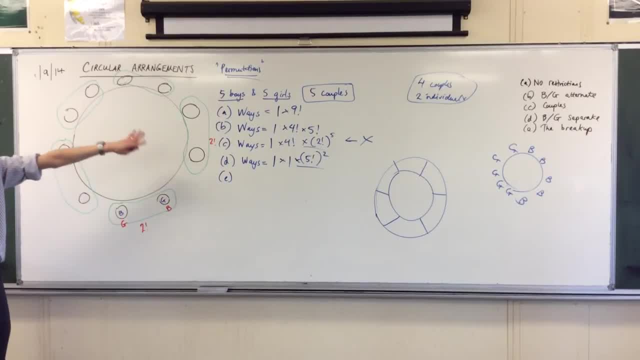 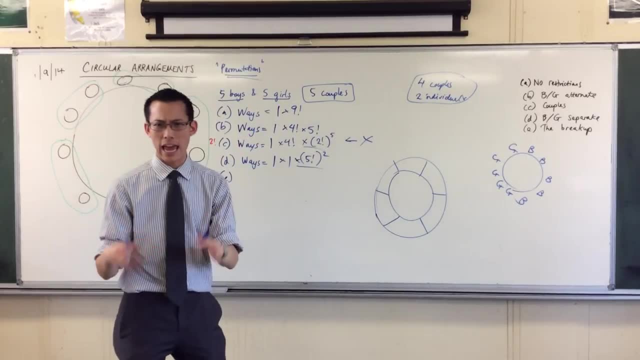 There you go. It's a life raft Or six different spots for things to be put into. okay, Now, the reason why this is a powerful approach is because a lot of people have gotten sort of hamstrung over saying: well, you know, there's one seat here. 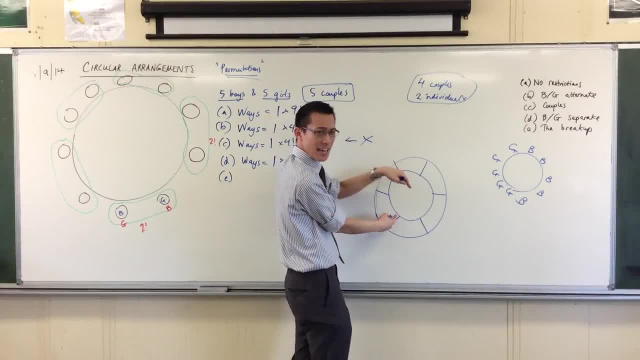 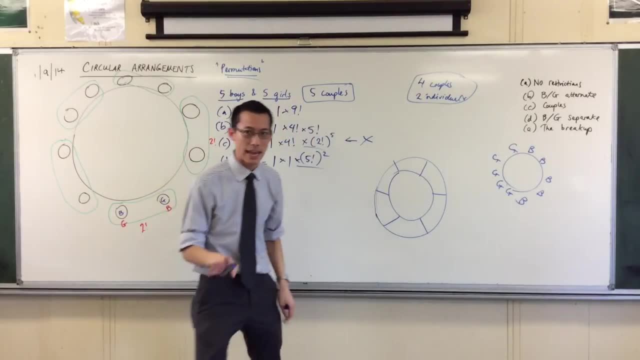 which means there's got to be a gap of one seat, or there might not be a gap of one. there could be a gap of two seats or three, or it gets a little more confusing, Can you see in this arrangement? I don't care about where the individual seats are, okay. 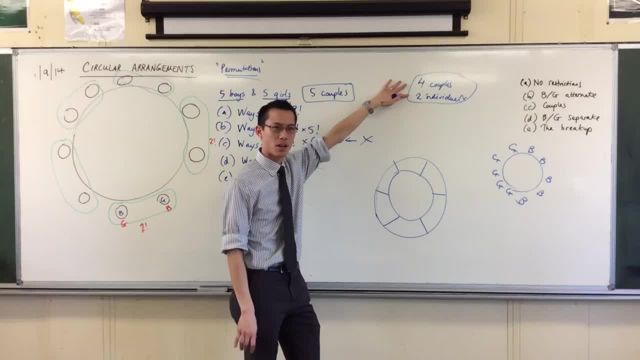 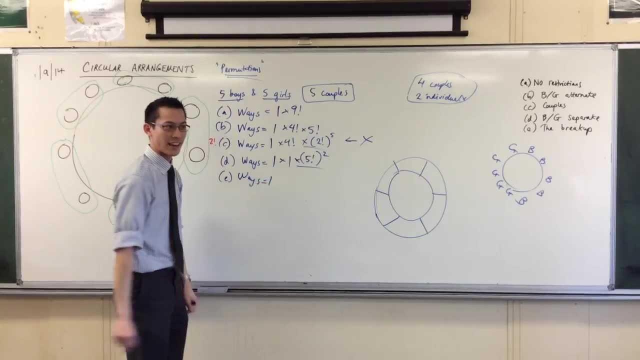 All I care is about where these guys are in relation to each other. okay, So I begin the way I usually do, by fixing someone in place. okay, So let's put the boy here right Once I've placed the boy, okay. 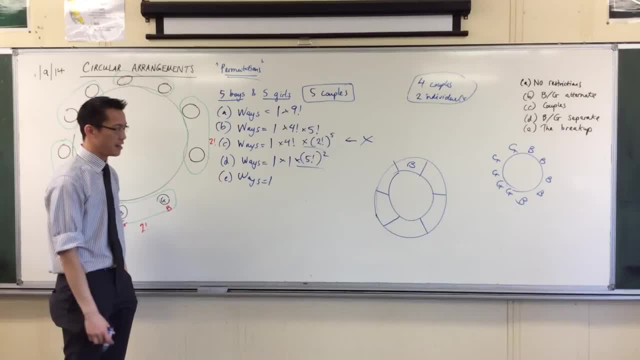 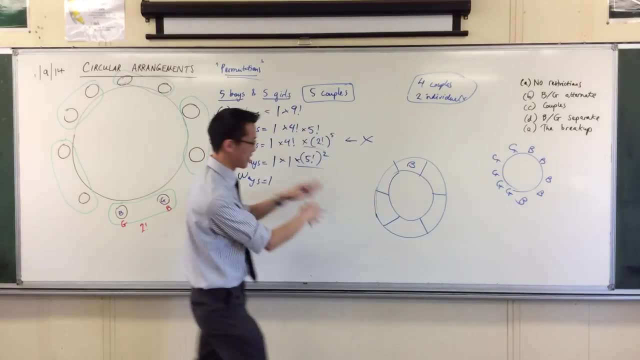 the girl is now limited in where she can go. right Now you can think in terms of: oh well, I have to put a couple here and here I prefer- and I think it's probably like mathematically easier to say: 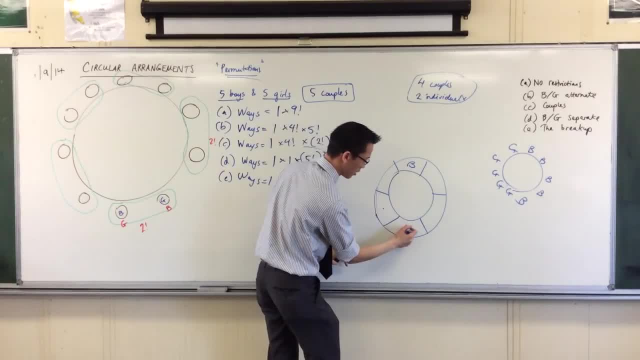 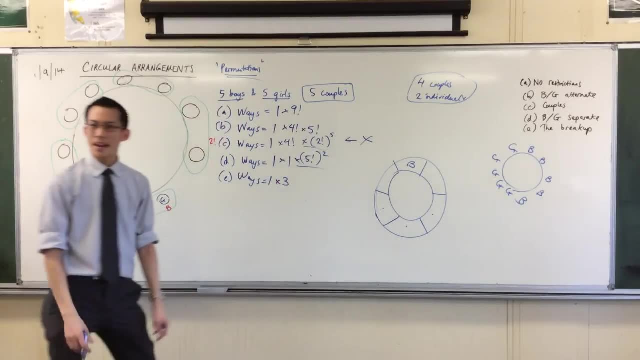 well, where can the girl sit? And the answer is here, here or here. There are three places that I can put the girl. Okay, now, once I've placed them, I don't care where anyone else goes. I just rearrange all the couples wherever. 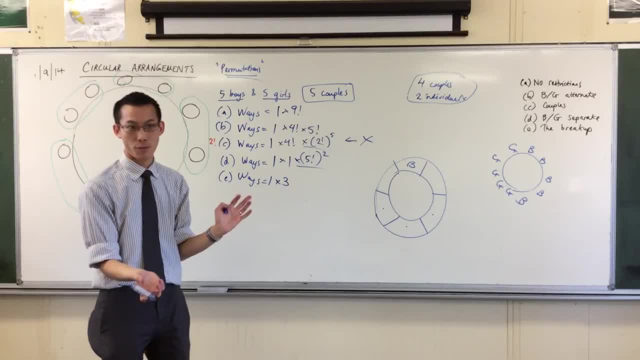 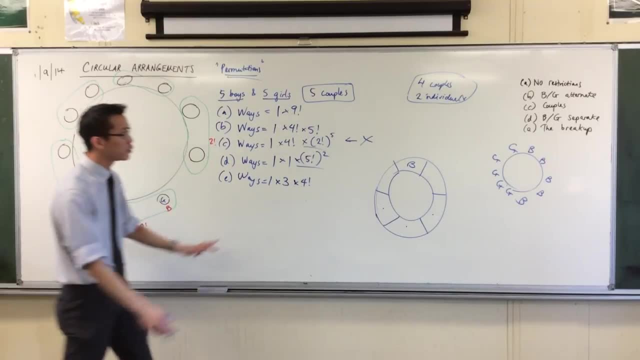 How many couples must I arrange? Four, And there are four factorial ways to arrange them. yes, Okay, now I'm almost done. I've put all of the units in their place now. okay, But then you know how formulas like they alternate. 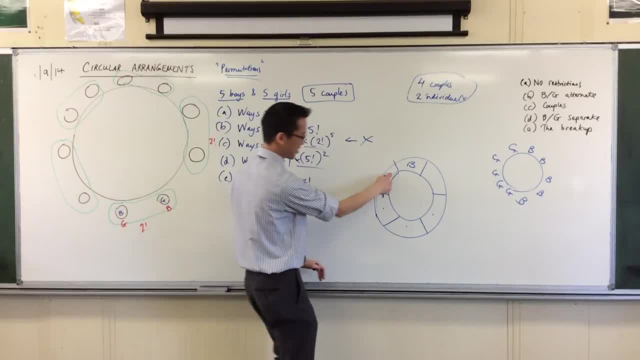 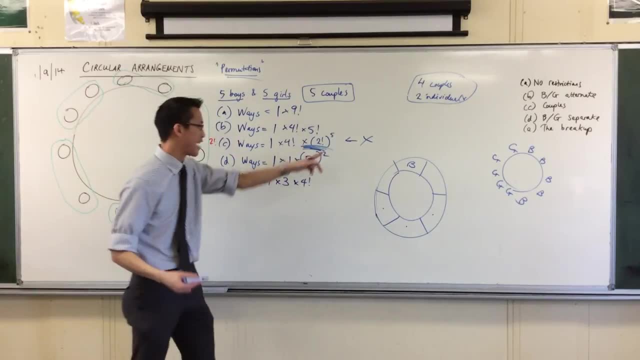 who gets beef and chicken or whatever. and, like you know, one of these girls is like: I don't want beef. So you know they swap places. So we can do all of this shuffling right, But I don't have five couples, do I? 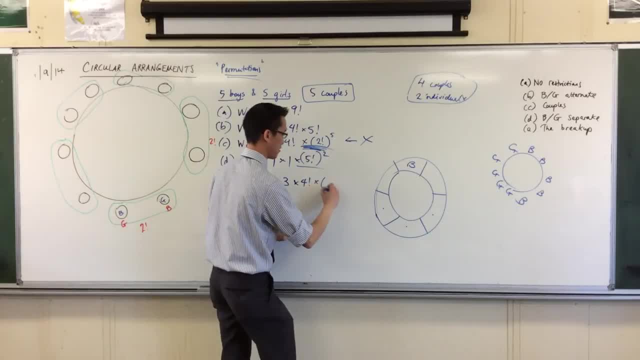 I've only got four right, Okay, which gives you. I think the number you end up with is 1,152, which is a bit of a relief, because, even though it's socially awkward, at least there's a 1,152 ways. 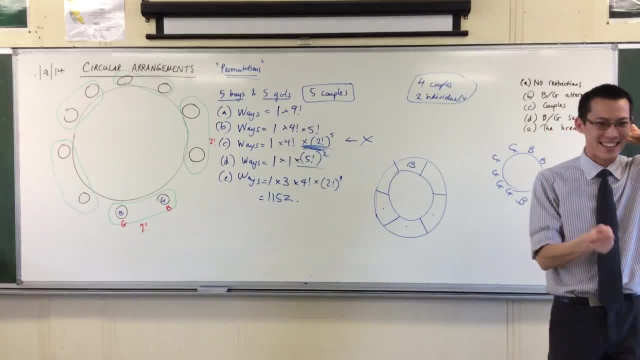 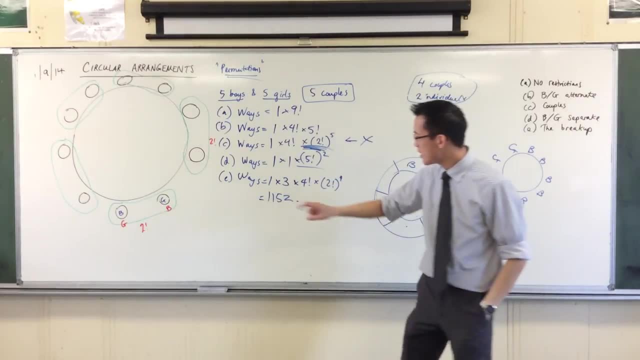 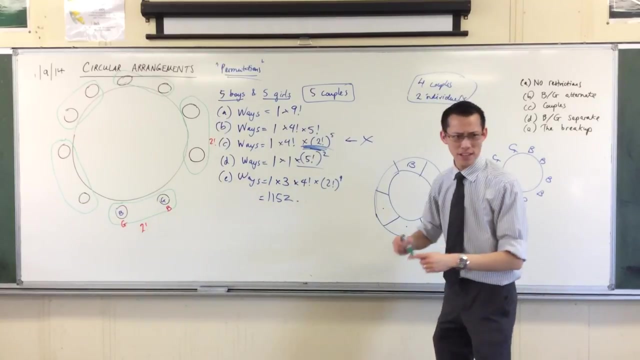 for us to minimize that awkwardness. Yes, You mean here. Okay, good question. Why is this not three factorial? Okay, Now, it all depends on- and I haven't written it, admittedly, but hopefully I talked through it slowly enough. 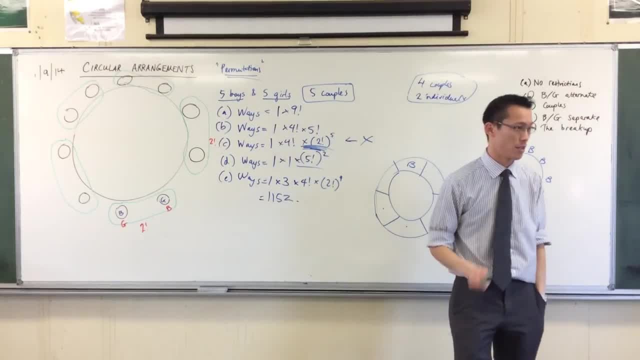 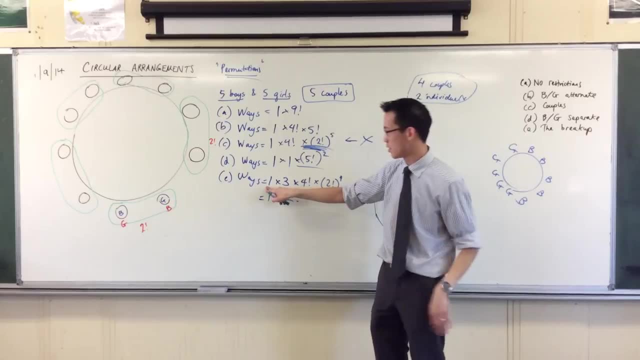 You've got to know what each of these means. Got it Know what each number means, right? So what was the one about? It was fixing a person, the boy in my case. okay, Then what was this for? And the answer was: 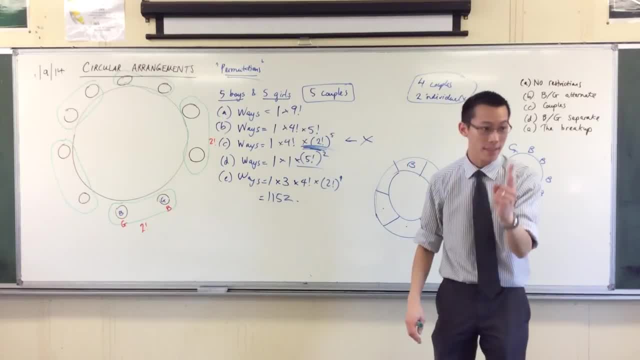 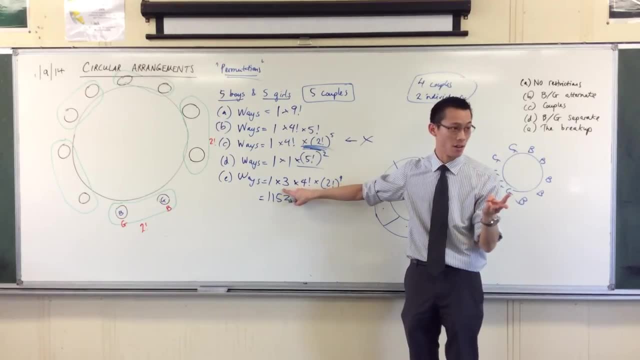 I was not arranging a bunch of things. I was arranging one thing: the girl right, And she can be in one of three places. There are three ways to place the girl right, So that's why it's three. Does that make sense? 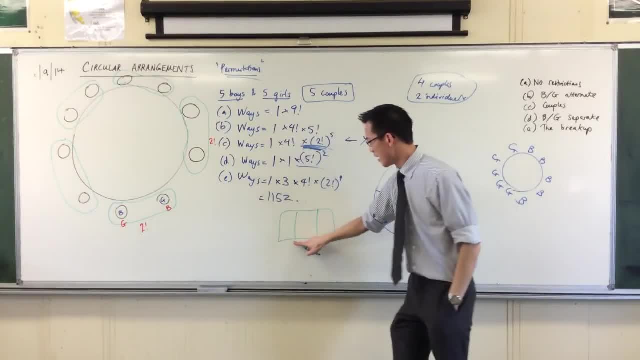 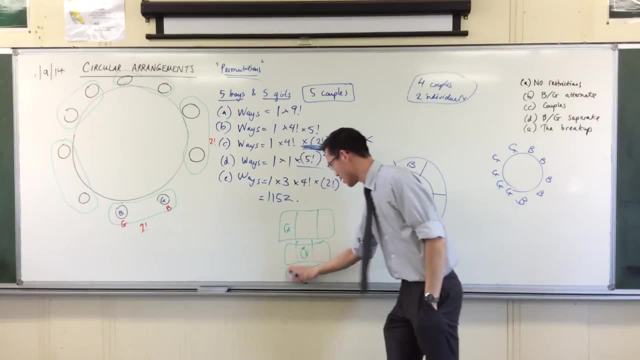 So if you want to think about it this way, right, Here are three spots, right, And the girl can be in this spot, or she can be in this spot, or she can be in this spot, And because I'm not placing three objects into those three spots- 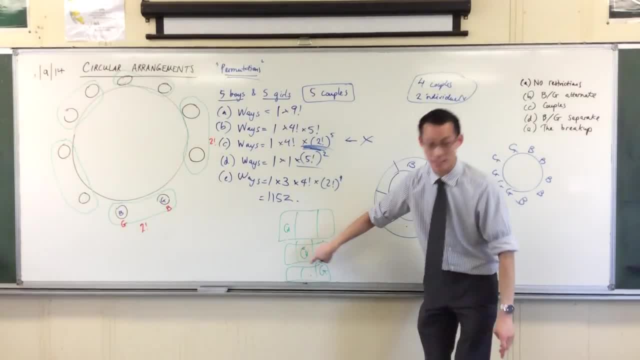 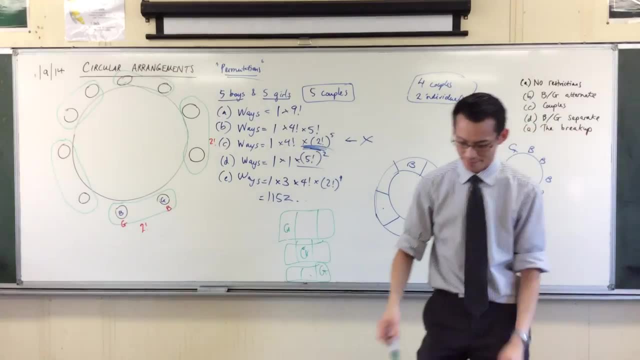 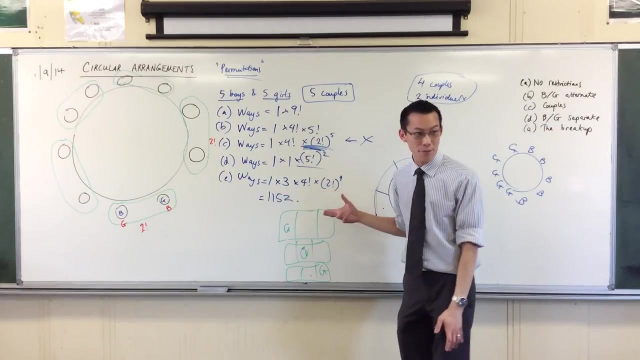 that's why I don't have three factorial. I'm only placing one object into those three spots. Make sense, Okay? So big tips: Draw a diagram for yourself, Know what each thing is there for right, And that way you can trace back if an error has crept in. 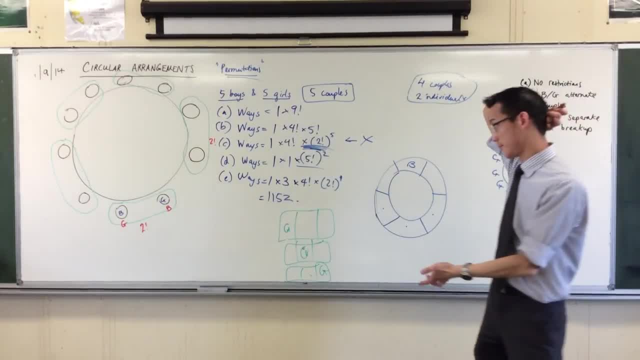 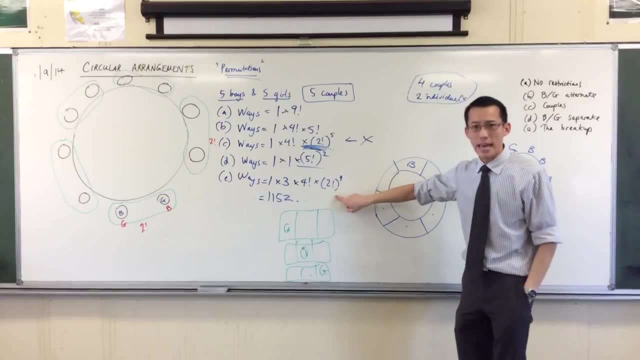 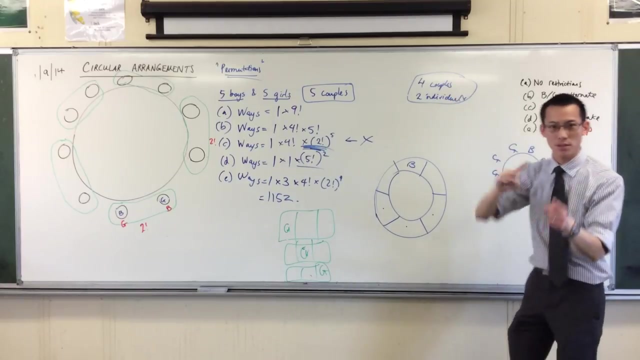 Yeah, What does this represent? What's this about? Okay, so this part is about after having placed the couples and then placed the individuals. Now I can see the couples themselves internally. they can swap. So there are only four couples though.